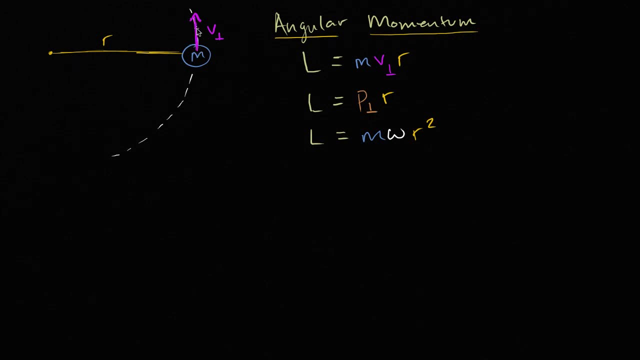 and let's say it has some velocity, And right here we have the magnitude of its velocity in the direction that is perpendicular to the wire that is holding it, or I guess you'd say perpendicular to the radial direction. Now, based on that, we've had a definition for angular momentum. 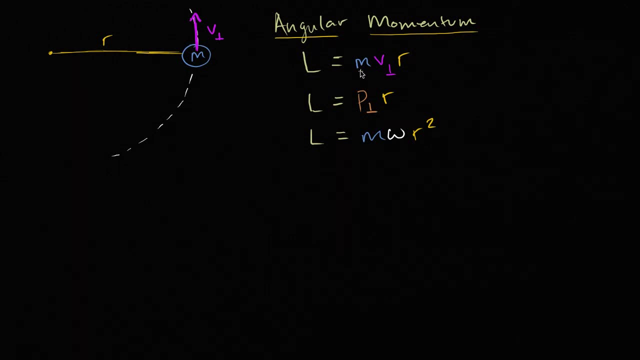 The magnitude of angular momentum is going to be equal to the mass times. this velocity times the radius, And you could also view that- and this is kind of always tying the connections between translational notions and rotational notions- we can see that angular momentum could be the same thing as 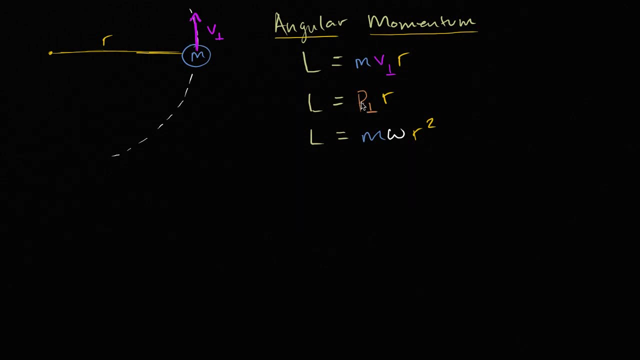 well, the mass times, this velocity. you could view that as the translational momentum rho, the magnitude of translational momentum in this direction times r. So once again, we took the translational idea, multiplied it by r and we're getting the rotational idea. 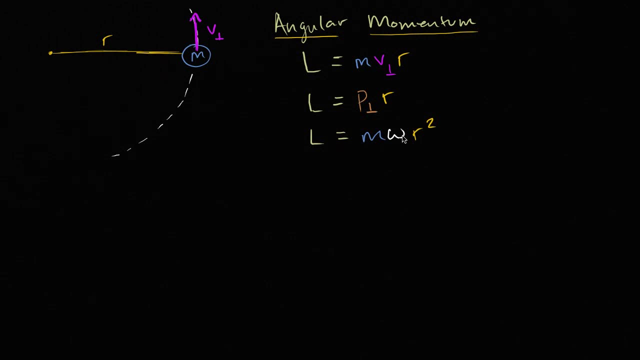 the angular momentum versus just the translational one, And we could also think about it in terms of angular velocity. and this comes straight out of the idea that this v is going to be equal to omega r. So you do that substitution, you get this right over here. 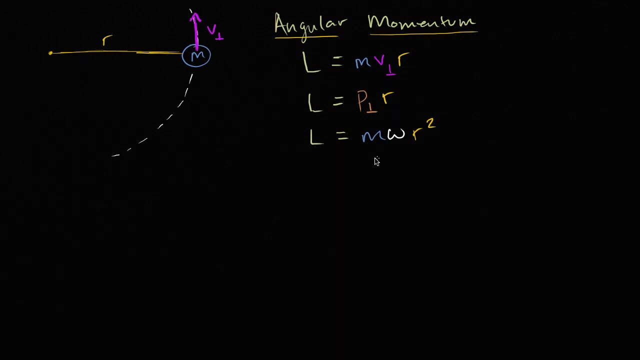 Now, in previous videos we said: okay, based on this and based on the idea that if torque is held constant, then this does not change, you can describe or you could predict the type of behavior or explain the behavior that you might see. 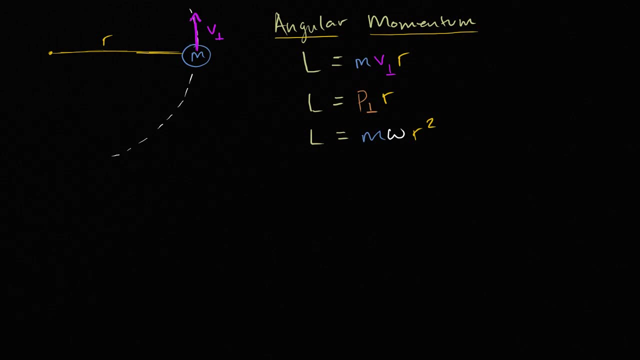 at a figure skating competition where if someone pulls their arms in while they're spinning and they're not, you know, applying any more torque to spin if they pull their arms in, well, if this thing is going to be constant, because there's no torque being applied, 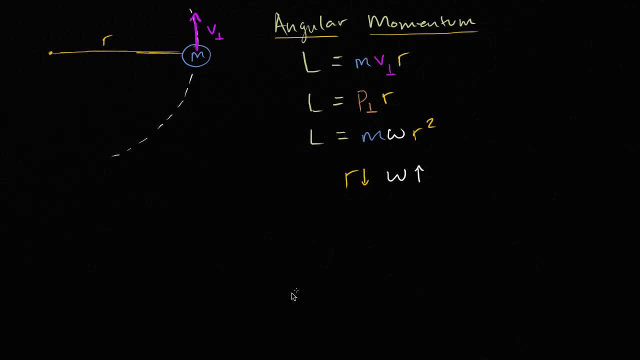 well, their mass isn't going to change, so they'll just spin faster And you do the opposite. the opposite would be happening, But you might have been left a little bit unsatisfied when we first talked about it, because I just told you that. 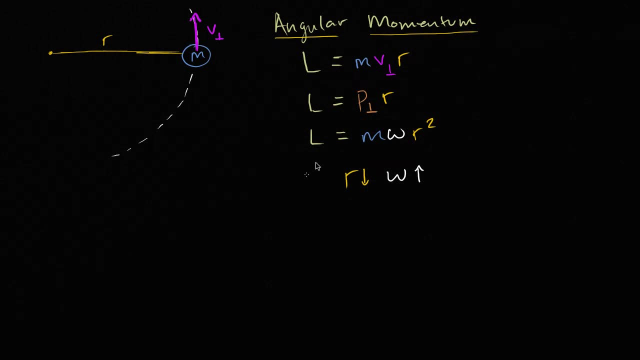 I said: hey look, if torque is, if there's no net torque, then angular momentum is constant and then you have this thing happening. But let's dig a little bit deeper and look at the math of it so you feel good that that is actually the case. 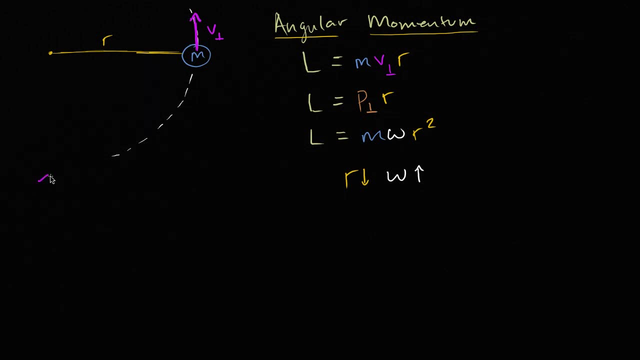 So let's go back, let's go to the definition of torque And so the magnitude of torque. I'll focus on magnitudes. in this video, the magnitude of torque is going to be equal to. it's going to be equal to the magnitude of the force. 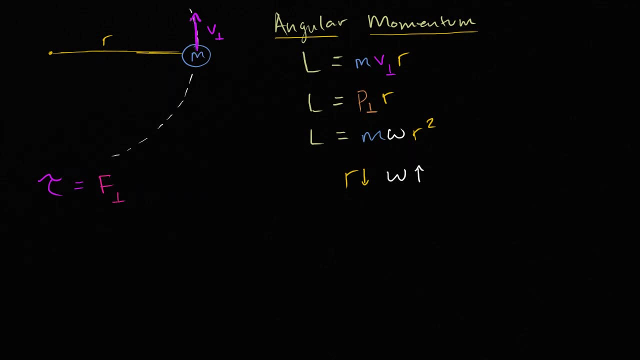 that is in this perpendicular direction: times r, times r. Now, what is this, this force? Well, this is just going to be equal to the magnitude of the mass force. F equals ma, So it's going to be mass times the acceleration in this direction. 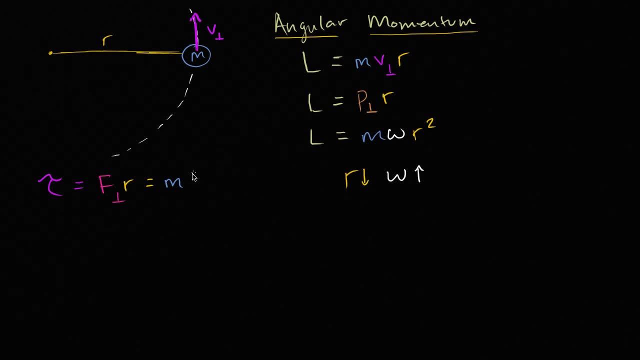 which we could view as, which we could view as the change in in this velocity over time, And we're talking about magnitude, so I guess you could say the magnitude of the velocity in that direction, And then, of course, we have times r. 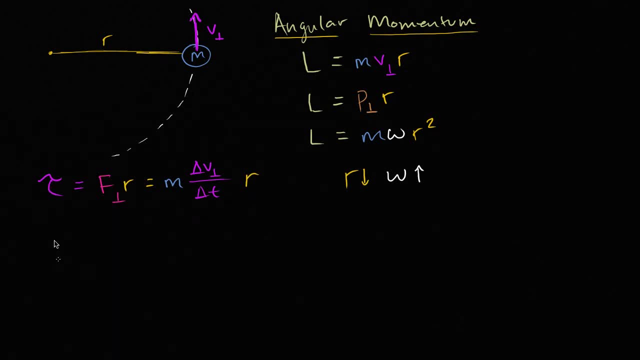 Times r. Now if we multiply both sides of this times delta t, we get, we get. and actually let me do tau in a different color- We do torque in green, We get. torque times, delta t, torque times delta t is equal to, is equal to. 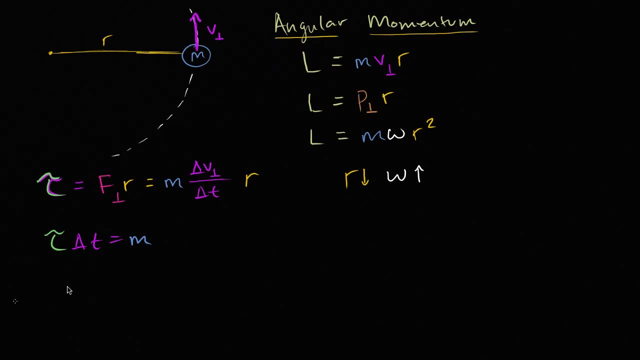 mass times: delta v, delta v in that perpendicular direction. times r. Well, what's this thing going to be? What's this? Well, that's just change in angular momentum. So this is just going to be change in angular momentum. 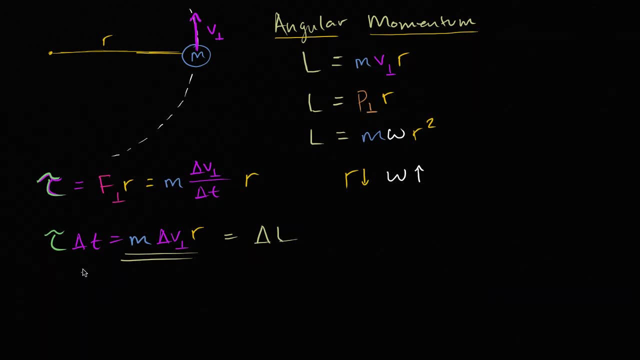 And there's a complete analogy to what you might remember from kind of the translational world. In the translational world you have this notion: If you take your force and you multiply it times how long, you're applying the force Actually. let me do this in a different color. 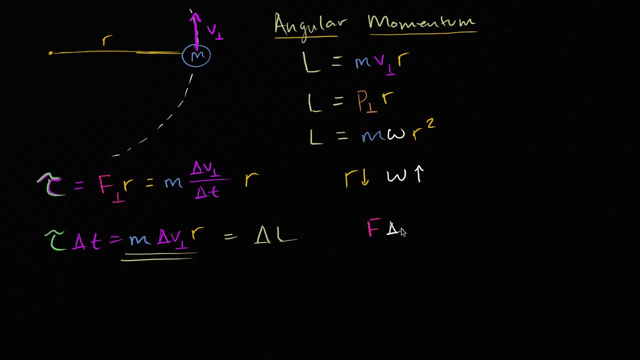 So you multiply it by how long you are applying the force. So this quantity we often call is impulse. Impulse, That's going to be equal to your change in translational momentum. Your change in translational momentum, And if you have no force, 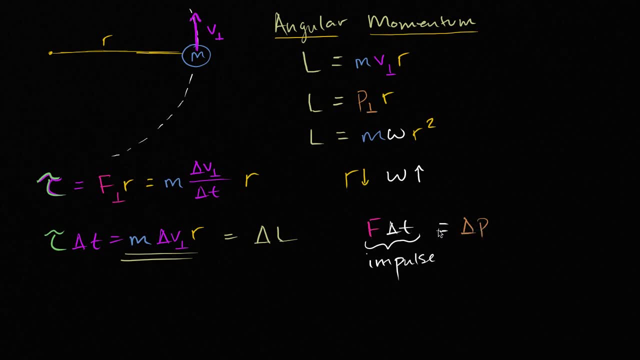 then you're not going to have any change in momentum, Or you're going to have your conservation of momentum, Or it's not going to change, It's just going to be conserved. And then you can do all sorts of neat you know: predicting where a billiard ball.